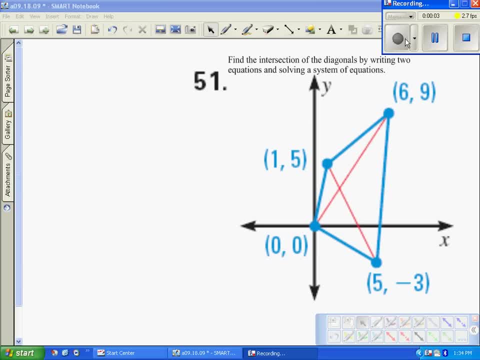 Given a quadrilateral, we would like to write two equations for the diagonals and solve a system of equations to find the intersection of the diagonals. We're going to start using the point 1, 5, and 5, 3 as two points on the line. Using those two points, we should 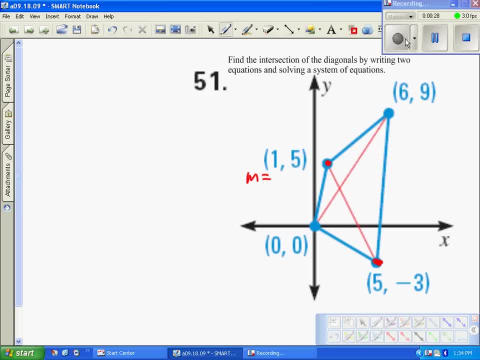 be able to find the slope of that line. We know 5 minus a negative 3 over 1 minus 5 gives me 8 over negative 4, which is negative 2. Now using that slope in this point, 1, 5, I. 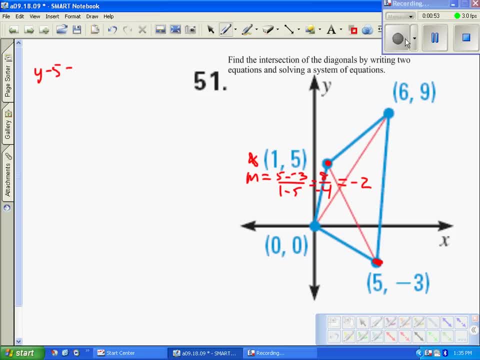 can write the equation: y minus 5 equals negative. 2. y minus 5 equals negative 2 times x minus 1. Distribute the negative: 2. y minus 5 equals negative, 2x plus 2 plus 5 plus 5.. y equals negative 2x plus 7 is my first equation. My 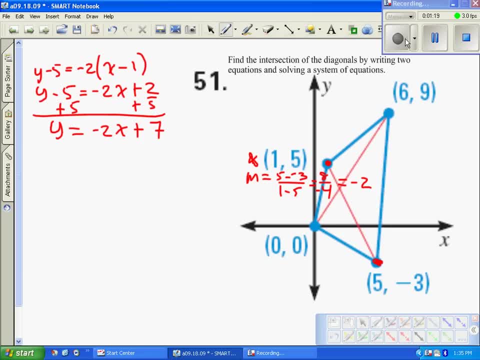 second equation comes from the point 0, 0 and 6, 9.. This one, we can find our slope, We can subtract: 9 minus 0, is 2, times 1, which is negative: 1 over 6 minus 1.. i seems. 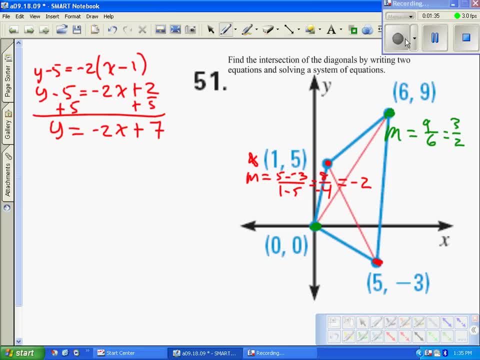 pretty convenient, because right now I have 6, half of 2 within 2, so out of that I have 6 over 9.. And now that we have our slope, we're going to subtract our t line, which is 2 times 0, 9, minus 0.. This is the first injustmin that we're going to do here. We 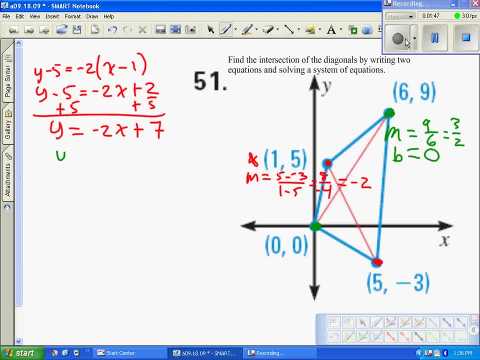 take that t line and we subtract t line and we schedule that t line. first- The last justmin is from the point 0, 0 into negative 2, and then we schedule the t line both times. Now when we do minus all and g this we do twice, 2 times minus 2.. Then we subtract the 2 to 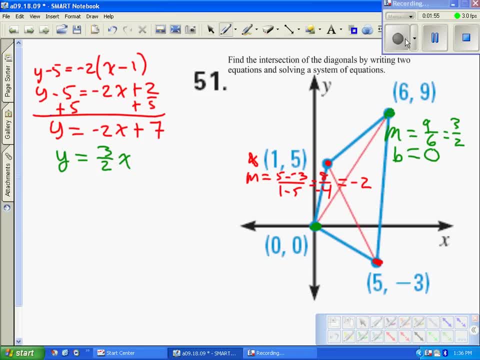 minus 0 and we campo them all. Then we execute the last justmin, asimizi to 19.. The next is, and is legal by subtractść: have a system of equations. I'm going to solve that by substituting for y and we're going.